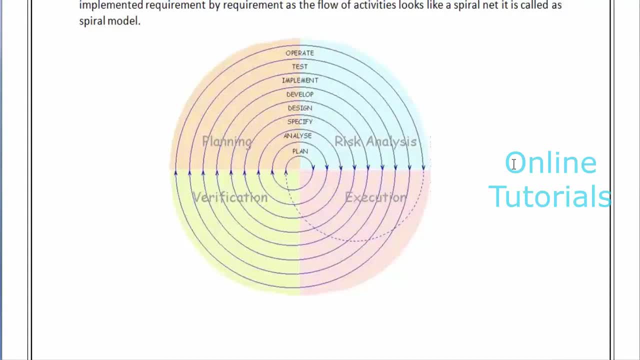 Before going to start a band They need some application, right? Yeah, they are. each of the company means it is a initial level, right? means, according to the Market levels, they have to give more features compared to to the other bands. Then only the particular band will be get famous, or otherwise, the more customers will come to the bank, right? 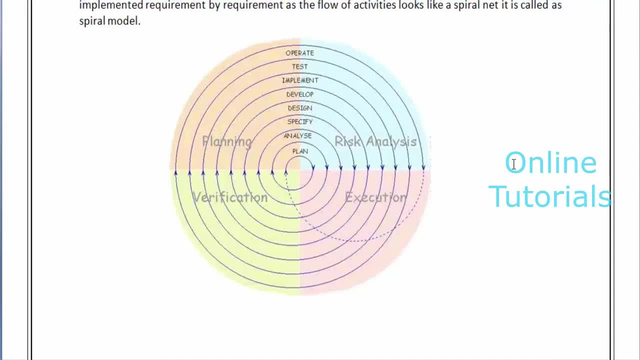 Correct. Yeah, at the point of time, according to the functionalism, while they are developing, the particular Modifications will come in a sequential way. right, means after one month, while they are developing the particular application after two months. okay, some other implementation will come to the Application related to other applications. nothing, but I see as a bank introduced one more option in their particular band. 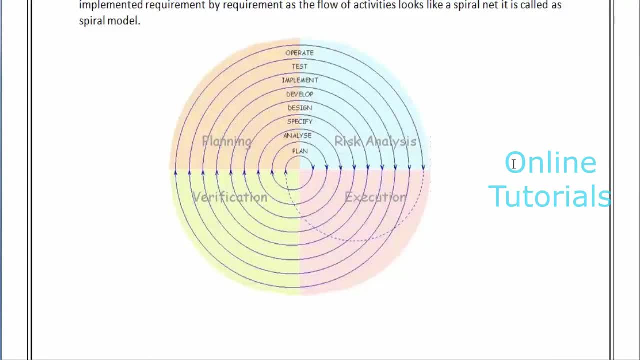 and The particular access bank has introduced one more plan to the customers. to attract the customers They introduce some other plan in a particular bank means the change is according to the market, changing market strategy, changing their how to change the application. because they are want to Establish the new bank They have to. 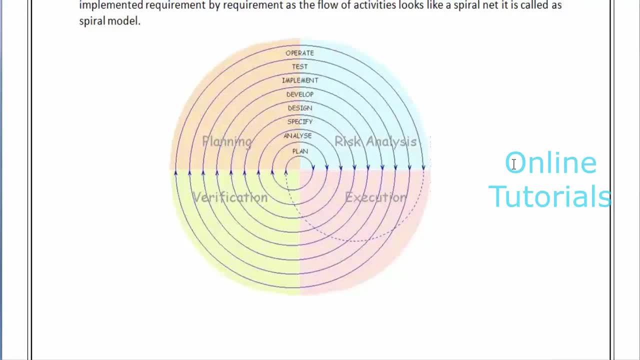 means give the competition To the particular existing come bands. then only the customers will come to you, other than the die existing fans. Right, Correct, Yeah, Yeah, at that point of time in the requirements will add day by day, right, According to the market changes, they have to add the functionalities every time and they have to remove the functionalities at the point of time, right. 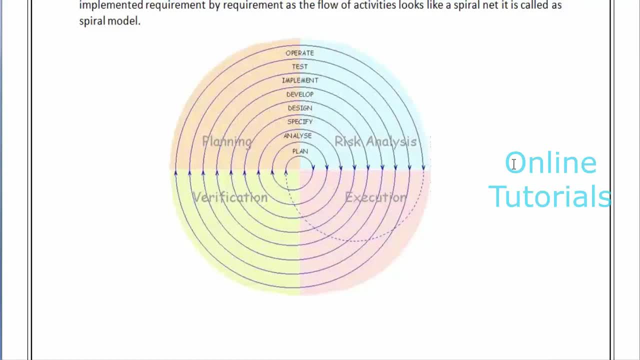 Correct for that time. There, the requirements are changing frequently. Okay, Okay, at that point of time, either model will be useful at that point of time. Okay, the festivals taken a tail. Okay, the festivals come, will come into the picture. Otherwise, anything will. any offer will come into the picture every time. the offer will not be available for lifetime, right? 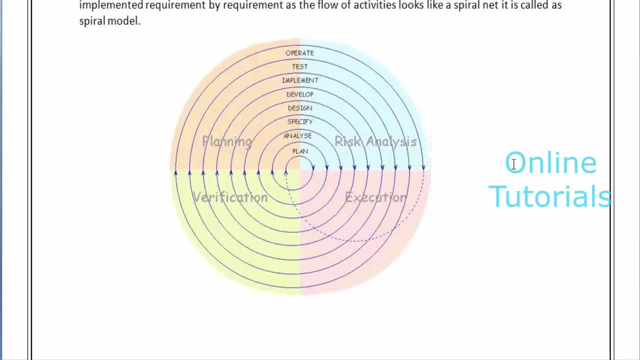 Okay, they will put some period of time from February 1st to January 2nd- Sorry, February 1st to March. that Okay, please. in this period They want to run one plan, new plan. They haven't as you have customers. Okay, means this is the new plan to the new customers. are the existing customers. means that the plan will be applicable for only for the particular.